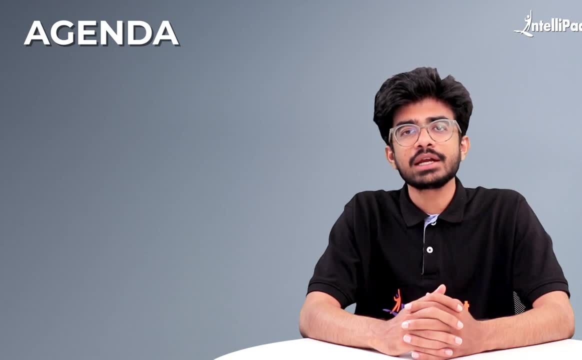 Now let us take a look at the agenda for the video. Firstly, I will be explaining about the introduction to distributed systems. We will be taking a look at the history of distributed systems, followed by what exactly is a distributed system, And after that we will be taking 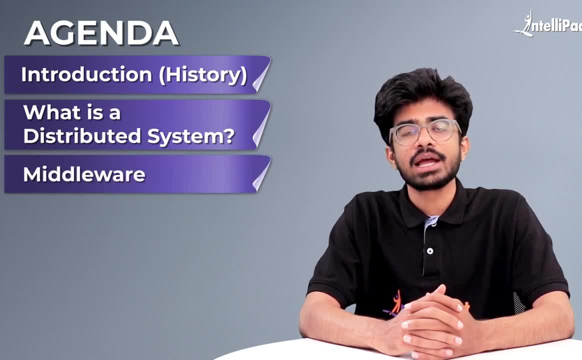 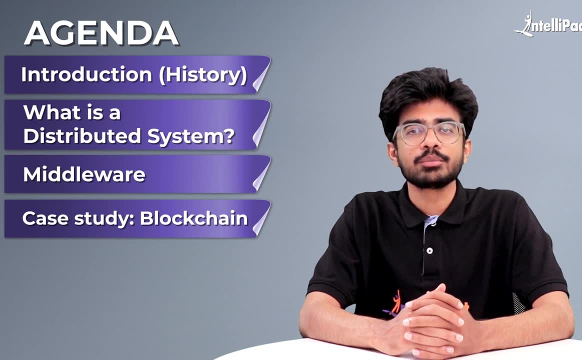 a look at a concept called middleware in distributed systems, And after that, we will be taking a look at a case study, which is for blockchain, And after that we will be taking a look at certain pros and cons of distributed systems, And after that, we will be taking a look at. 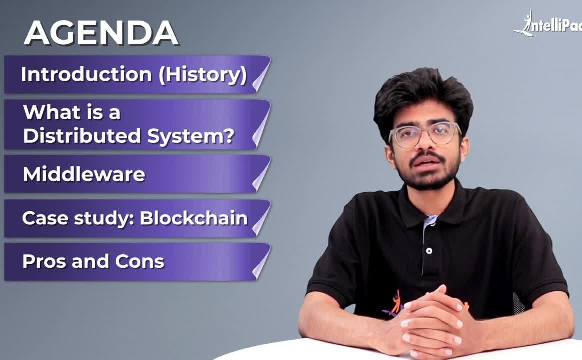 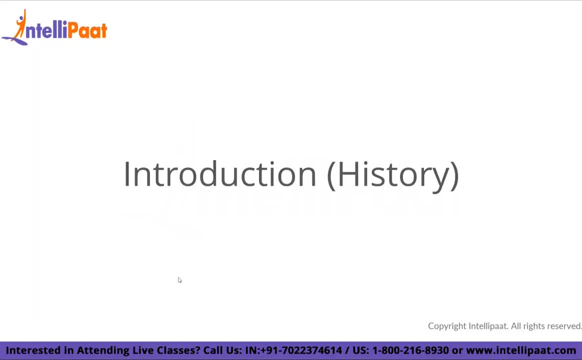 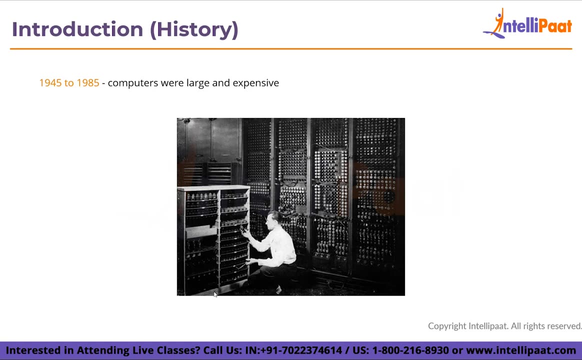 the most basic theorem in distributed systems, which is the CAP theorem. Let us move on to the first topic, which is introduction. So since the 1945 to 1985, computers were generally very large and expensive, as you can see in the picture below. So it needed. 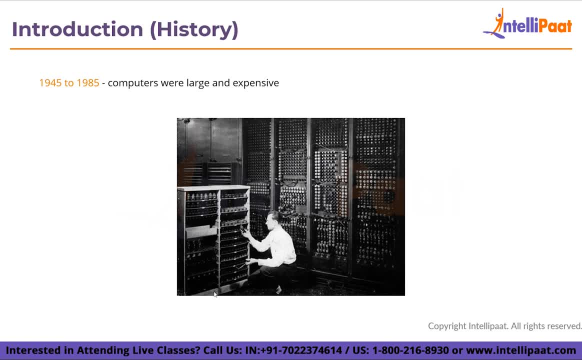 a whole room to just have a basic working computer. So the early day computers, or the first generation computers, they use something called vacuum tubes, And vacuum tubes were very large. they were used to store data and make computations on this data. So, as you can see, they were very large and it needed a large amount of 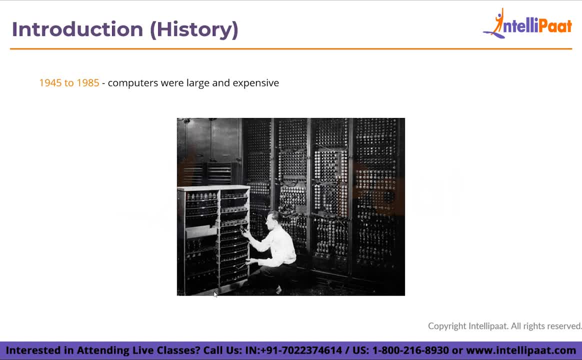 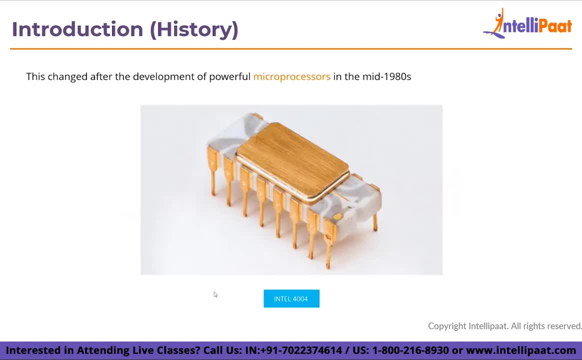 them, the olden day computers. they needed a large amount of vacuum tubes to do the basic tasks. So, and then after that, all of these things changed after the development of a powerful microprocessor. What you see in the image is the Intel 4004.. It was among one among the early microprocessors to be developed. 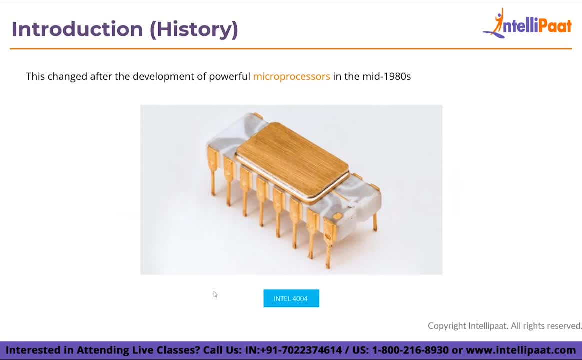 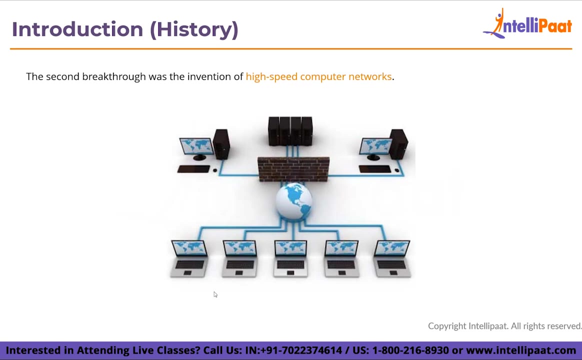 This started in mid 1980s, 85,, 86, and so on. So every major company started manufacturing microprocessors. So the size of the computers generally became smaller after the invention of microprocessors. And this was the first breakthrough, that is, the invention of microprocessors was the 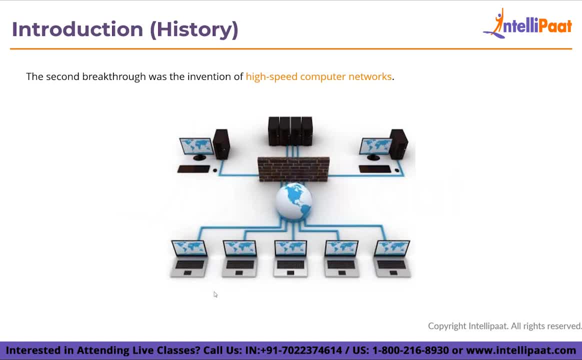 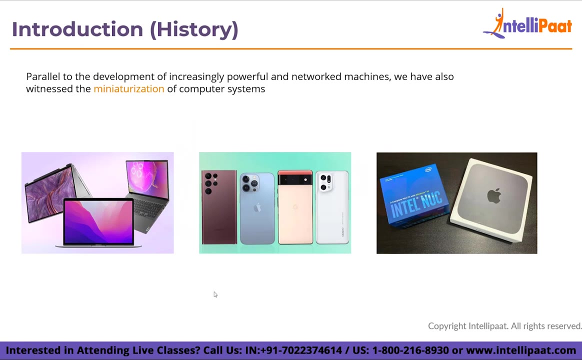 first breakthrough in computing And then the second breakthrough came when the invention of high speed computer networks took place. And parallel to this, parallel to the first and second breakthroughs, we had another breakthrough. You cannot call it as a breakthrough, it is. 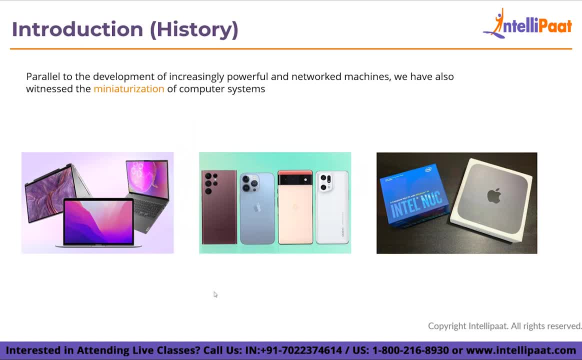 just called as an evolution of the computers, due to the result of these first and second breakthroughs. So what was this byproduct of the evolution? This was the miniaturization of computer systems. So in present times- in 2022, we can see laptops, we can see tablets. 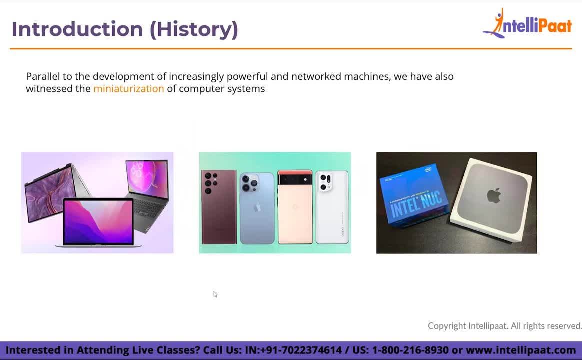 and we can see hybrids between tablets and laptops And you can see top notch mobile devices, which is pretty much its saturation, Like we have almost perfected the smartphone industry right now. And then you also have portable desktop, portable computing, like the Mac Mini and the Intel's NUC. You don't even have to own a desktop now, you can just. 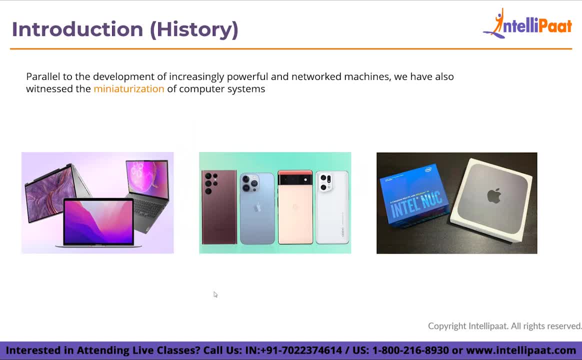 it will be a size of a power brick and you can just carry it and it will have all the slots. You can just connect your monitor, mouse, keyboard, whatever. then you can set up your desktop anywhere, so we have portable desktops as. 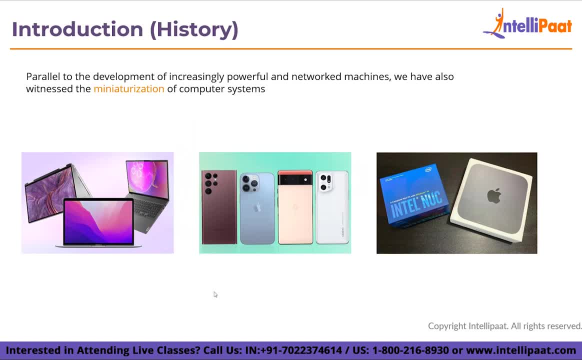 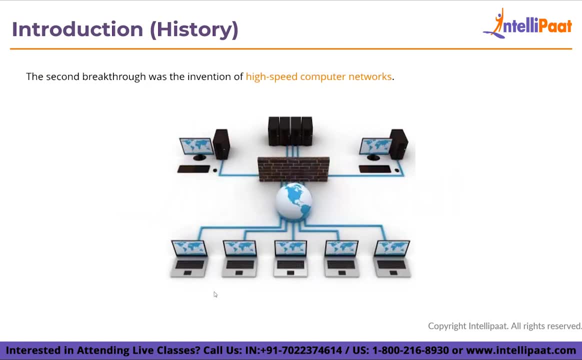 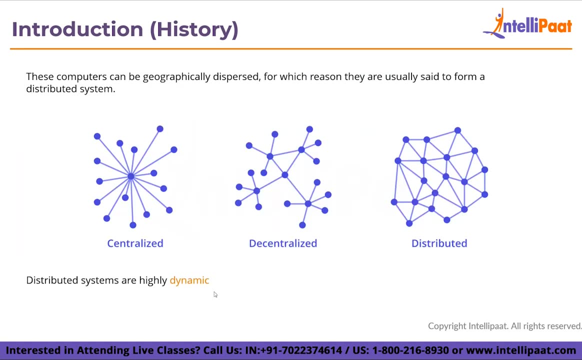 well, so we have all these miniaturization of all the computer devices and all the form factors. this was the result of high-speed computer networks and then or the invention of microprocessors. these computers, that is, the nodes, can be geographically dispersed, for which reason they are. 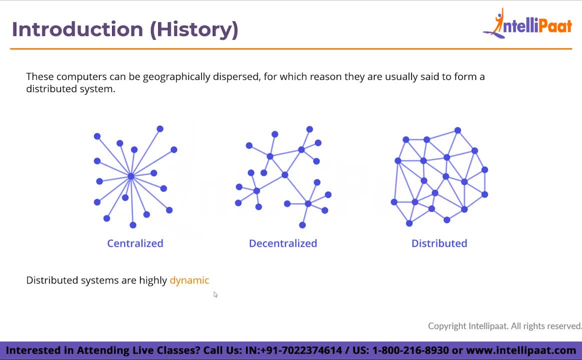 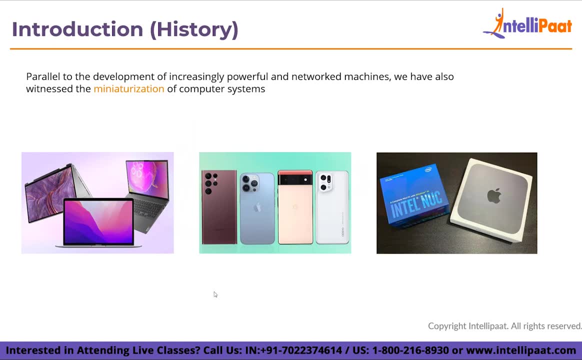 usually said to form a distributed system. all right. so because of all these three improvements, that is, the microprocessor technology, the networking and miniaturization of computers, it is now easy to put together a computer system composed of a large number of computer networks. so these computer 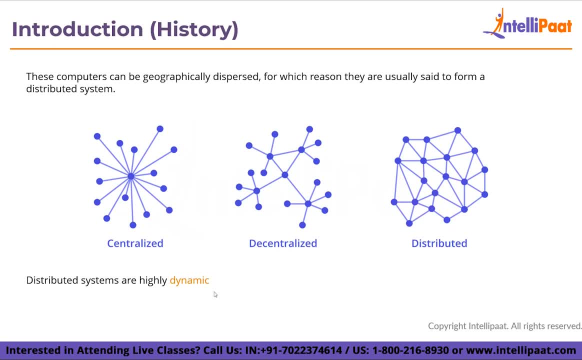 networks have nodes and these nodes can be geographically dispersed, for which reason they are usually said to form a distributed system system. we have the centralized network, computer network, or wherein one centralized server or a computer sits in at the center and then it is connected to every other node. when coming to the decentralized architecture, you have that. 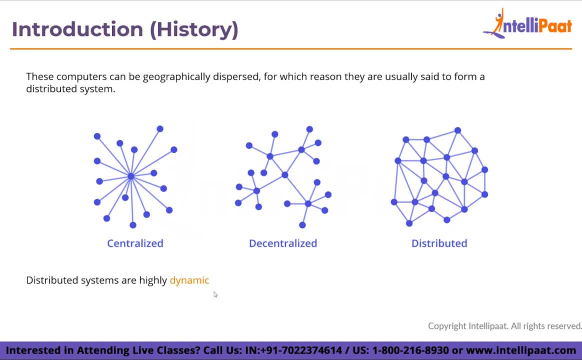 centralized nature is taken out and it is split into many central bodies and these central bodies will have connections- physical connections or wireless connections to other nodes. so basically, every nodes will be connected, but you will still have one node which is telling the other nodes what to do. 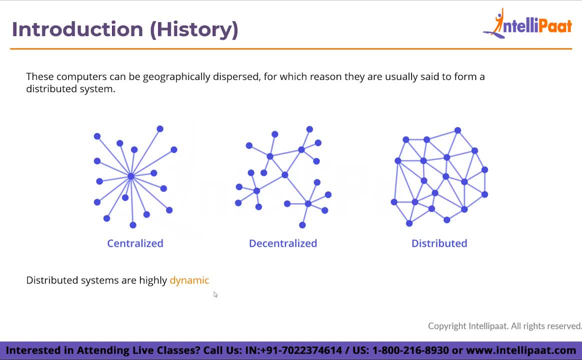 that is, in decentralized, you still have some form of control, you still have some form of centralization. but when it comes to distributed, every node is connected to every other node and every other adjacent node, and then no, no one owns the network and no one has control of the network. 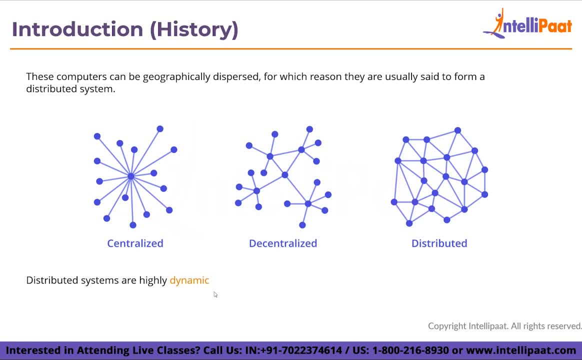 basically, every node is given equal rights. so this is what distributed means, and one more point i have to add here is that distributed systems are highly dynamic. now, what do you mean by dynamic? it means that computers can join and leave, and they can adapt to changing topology and performance. 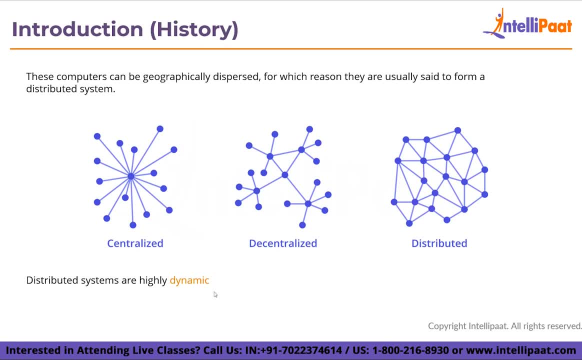 that is, any number of computers or nodes can be adjoin, can join the distributed network, and they can leave at any point. oh, this will not affect the overall network, and then each node can adapt to changing topology. topology here means the physical layout of the network and then performance. 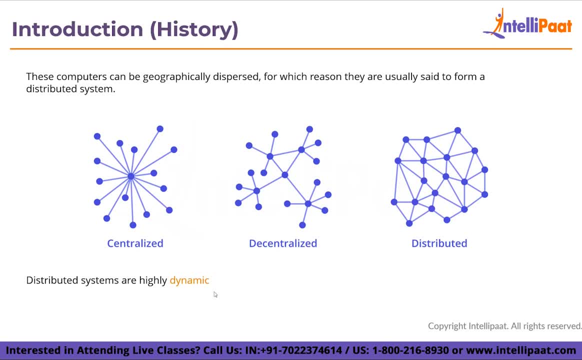 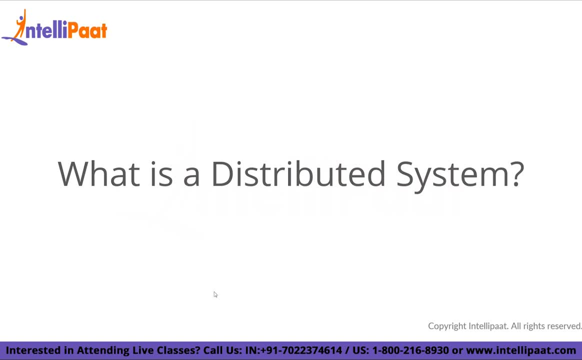 also, it can adapt to performance as well, so that is why it is called dynamic. now that we know how distributed systems came into the system, then we can also adapt to the performance of the network. now let us move on to picture why it was created and what are all the factors that caused the. 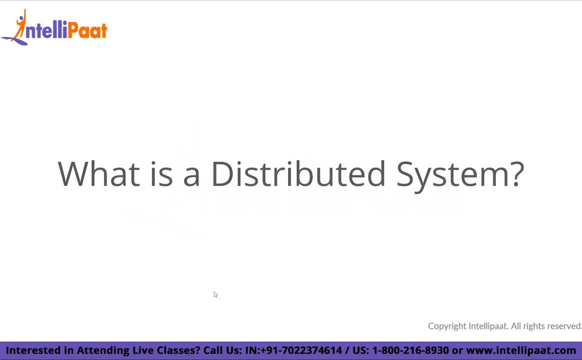 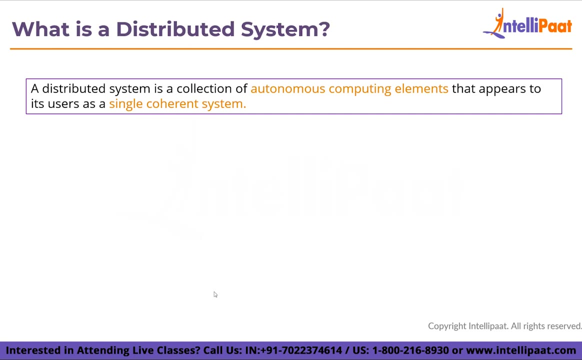 invention or the formation of a distributed system. now let us move on to the explanation, or we will see what exactly is a distributed system in this topic. now the formal definition of distributed systems go something like this: it is basically like defining a distributed system is very tough. 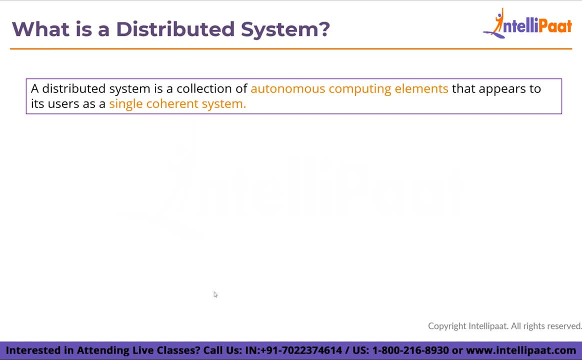 this is somewhat a loose characterization of what a distributed system is. so anywhere you find- even if you google what is a distributed system like, there is no hard and fast definition to it. so this is a loose characterization that is taken from one of the credible textbooks by Andrew Tannenbaugh. 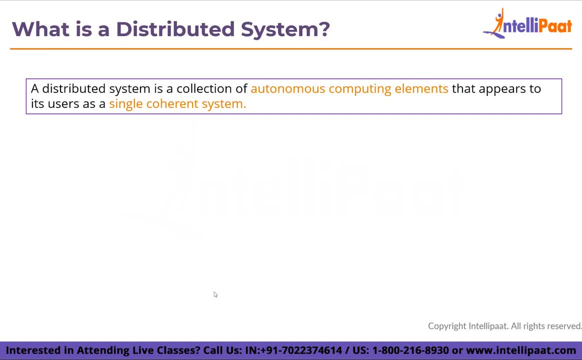 so he says a distributed system is a collection of autonomous computing elements that appears to its current system. now let us break down this definition. so basically this note: that definition refers to two characteristic features of distributed systems. so it says it is a collection of autonomous computing elements. what do you mean by autonomous computing elements? so autonomous means that it is independent. 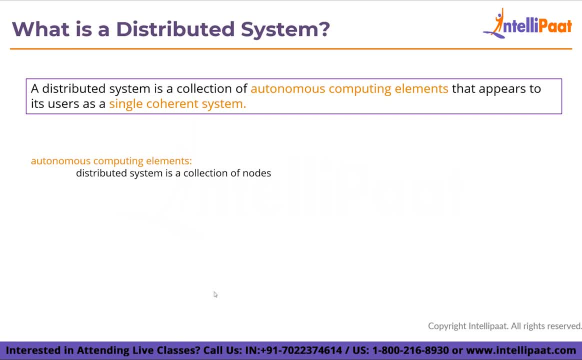 of other nodes in the network. that is, a single computer in the network can be independent of any other computers. so that is what you mean by autonomous, and computing elements is called as a node here. so the general term is node. a node can be a person using a computer, that is a user like using a 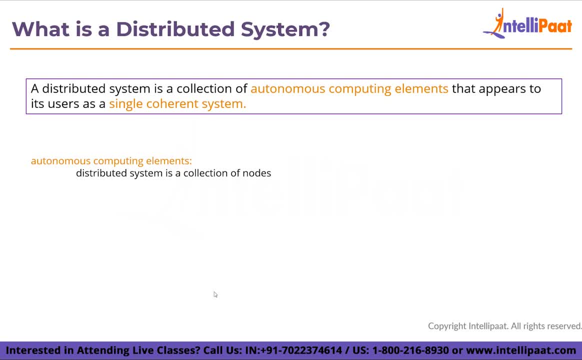 physical actual computer or a node can also be an application running in a computer. that is, let's say, if within a computer there are several applications running, so you will have to address each application as a node. and then the second characteristic feature that is defined in this definition is single. 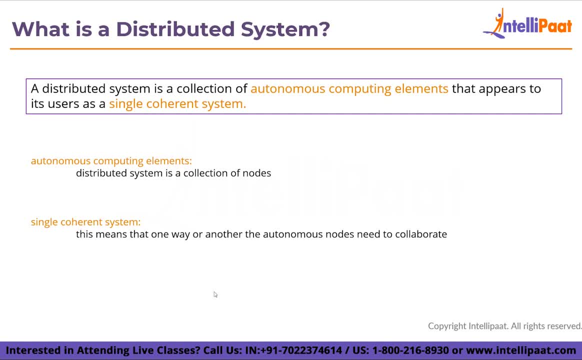 coherent system. now, what do you mean by single coherent system? this means that one way or another or the autonomous nodes needs to collaborate right. so in order for the user or to believe that the network is a single system, all the nodes within that distributed system needs to act like it is one system. so for that it needs to collaborate in some fashion. so this is: 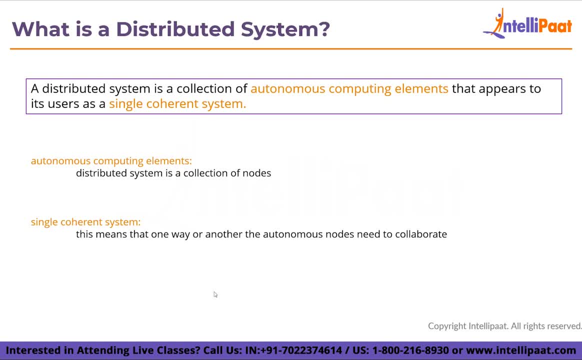 what it means by a single, coherent system. so let me give you some examples of a distributed system right now: Facebook. Facebook is a distributed system. blockchain technology- whatever the applications of blockchain is right now- is distributed systems, and then online multiplayer system is a distributed system, and then online multiplayer system is a distributed system and then online multiplayer. 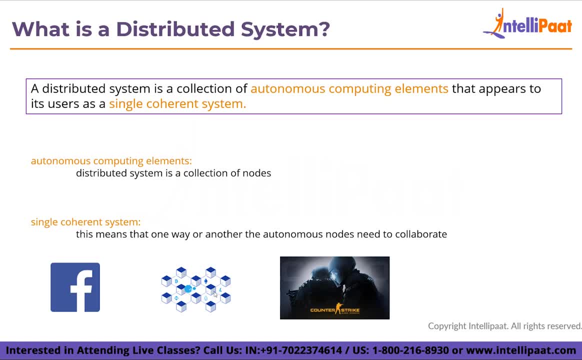 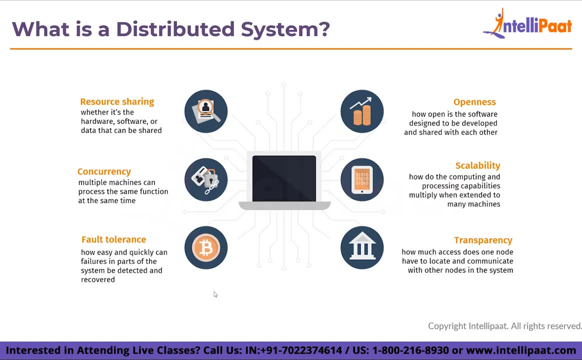 games like counter-strike, dota 2, etc. are all distributed systems. now let us go through some of the most important functions of distributed computing. let us see what they are. so the very first function is the resource sharing. so in order to be a distributed system, you will have to share. 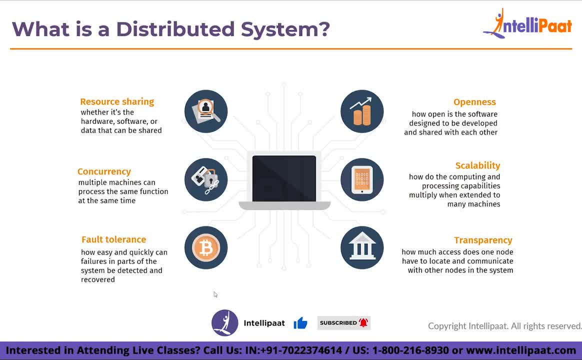 resources among other nodes, whether it is hardware, whether it is software or data, you, you will have to share your data among other nodes. so, in order to be a distributed system, you will have to share resources among other nodes, whether it is hardware, whether it is software or data, you, you will have to share. 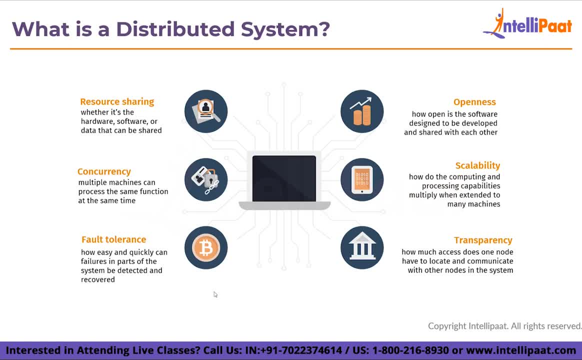 your resource, among other nodes, your adjacent nodes. and then the next feature or function is openness. openness here means that how open is a software designed to be developed and shared with each other? this means that if a software is developed by using the distributed network, it has to be open. there must be transparency in the software. and the next function is: 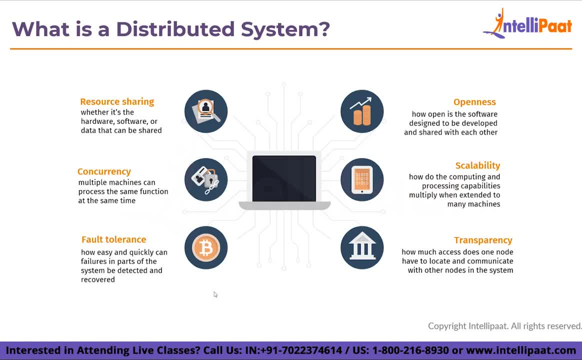 concurrency. concurrency here means that multiple machines can process the same function at the same time. so let's say you want, you are in a distributed system and one node is downloading something and some other node should be able to download the same thing at the same time. this is what you mean. 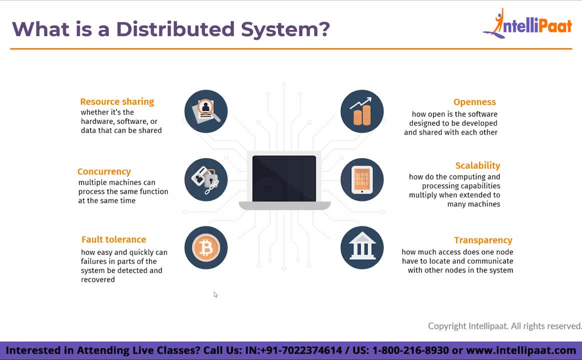 by concurrency. and moving on to the next function, we have scalability. scalability means how the computing and processing capabilities multiply over time, and how the processing capabilities multiply over time and how the when extended to many machines. so let me break this down. let's say you have a. you have 10 nodes. 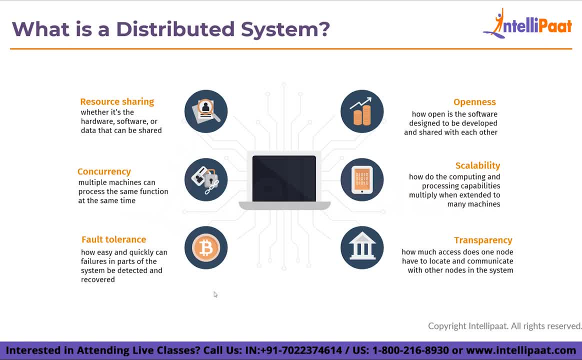 in a distributed network. you buy 10 nodes and then you form a distributed network through these 10 nodes. so you have a software. you create a software and you deploy it on the network- one of the nodes in the network- and everybody can access the software. now you want to increase the network. 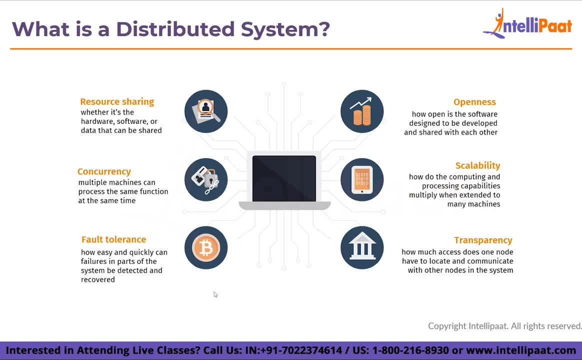 that is, increase the population of the network by adding in 90 more nodes. let's say now the node size, like the number of nodes in the distributed network, is a hundred. so now the software has to work in the same manner, that is, it has to give out the same functionalities in the same amount. 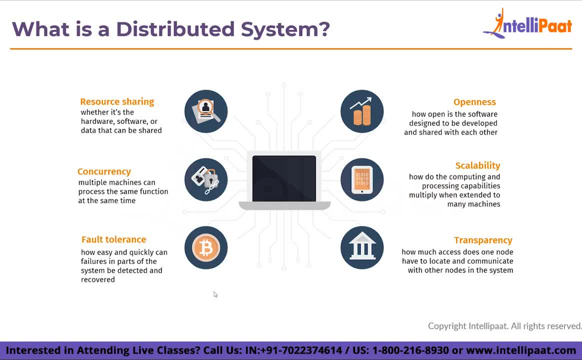 of time, with no lag, no issues, no latency, for the hundred nodes as well. so this is what you call as scalability. so this is one of the functions or features of distributed systems. next we move on to fault or fault tolerance. fault tolerance here means that how easy and quickly can failures in parts of the system can be detected? 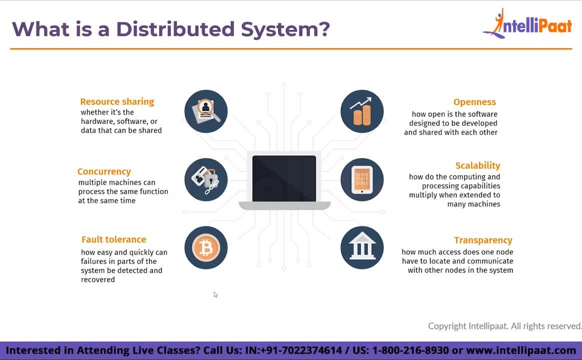 and recovered. so let's say, a system, a group of nodes go down and the data or software in that nodes should be duplicated in some other node so that you can, so that the data or the software can be retrieved. so fault tolerance is one of the features. and finally we have transparency. transparency here means that 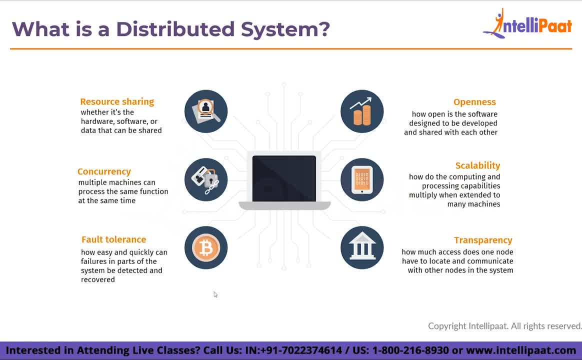 how much access does one node have to locate and communicate with other nodes in the system? so every node is treated as the same here. every node is allowed access to whatever data, whatever software, whatever hardware resource that is there in the distributed network. so it has to be. 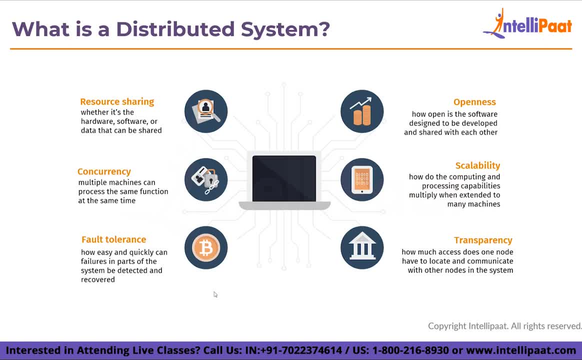 transparent. although you can give like, you can set user authentication or user access within the distributed networks, that is, you can cut off certain functions for a particular node or a group of nodes. that can be done through software, but generally a keyboard can be used for this, and that's why this can be the biggest challenge: our distribution. 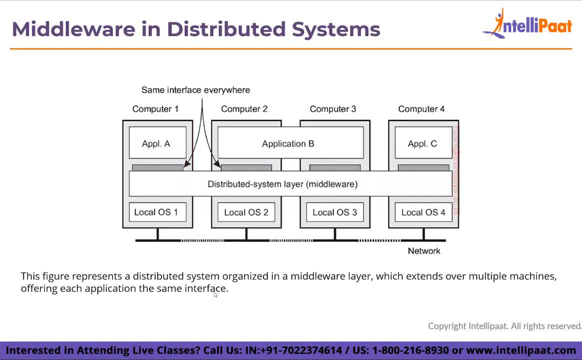 okay, so we are done with the textbook distribution. alright, now let's move on to the next section, which is middleware in distributed systems. all right, as you can see in the picture now, this picture is taken from the textbook distributed systems by andrew tannenbaugh, and this figure: 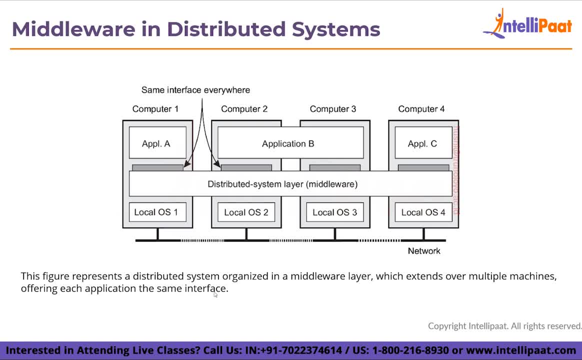 application, the same interface. now, when you look closely in the image or the figure, it shows four computers, that is computer 1, 2, 3 and of which application B. so you have three applications here: application A, B and C. and now application B is distributed across computers. 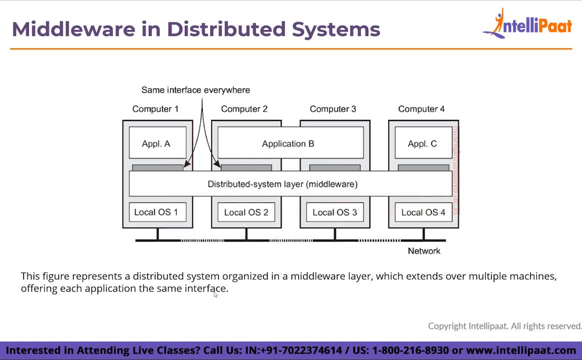 2 and 3. each application is offered the same interface, that is, application A, B and C communicates to the computer's or the nodes through the same layer, called as the distributed system layer or middleware layer. begitu distributed system provides the means for components, components or nodes of a single distributed application to communicate with each other, but also to 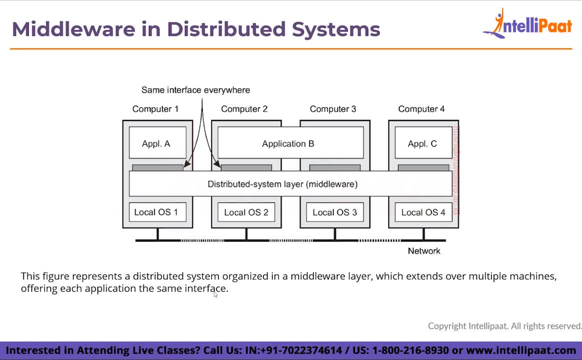 to let different applications communicate, that is, the applications can communicate between themselves when you have something called as a middleware layer. at the same time it hides as best and reasonably as possible the differences in hardware and operating systems from each application. so let's say a software engineer creates application a some other set of software. 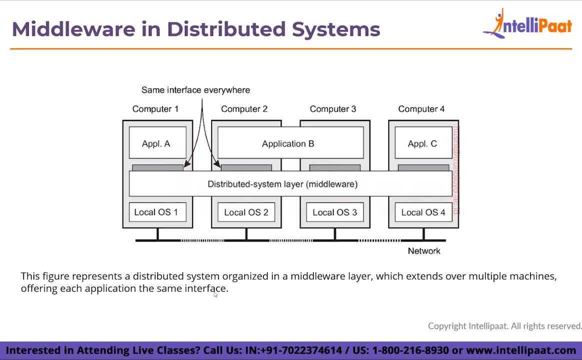 engineers create B and some other set of engineers create application C. so no us, now they have. they have to take into account each node. that is, each node might have a different operating system. they might have different hardware configuration as well, so this becomes very complex for the engineer. 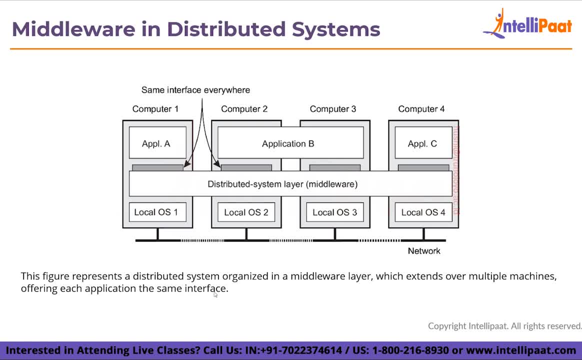 software engineers to develop applications which are especially catered to each and every node you. so, instead of that, if you put a distributed system layer or a middleware layer, they get. they should only worry about what the middleware layer is, what it brings to the table and what you. 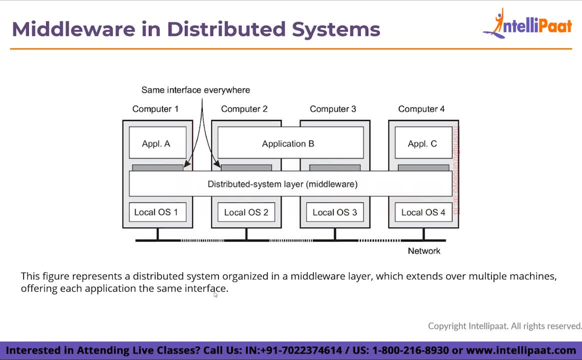 have to cater to the middleware so that you can communicate to the to all the nodes, so they only have to worry about the middleware rules and regulations, so that they can create applications without having to worry about the operating system and the hardware of each and every node. so this is why you need something called as a middleware. 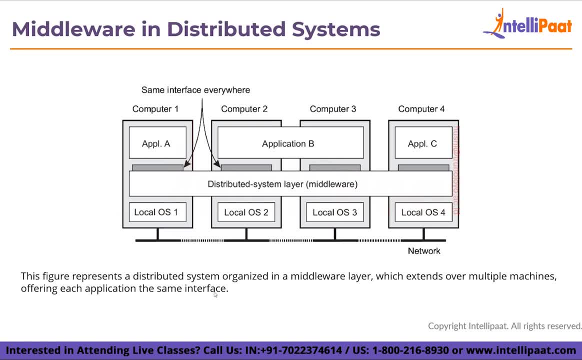 in a distributed network. in a sense you can also say that middleware is the same to a distributed system as an operating system is to a computer. it is a manager of resources, offering its applications to efficiently share and deploy those resources across a network. so he's saying that he is basically paralleling out the middleware and the operating system. 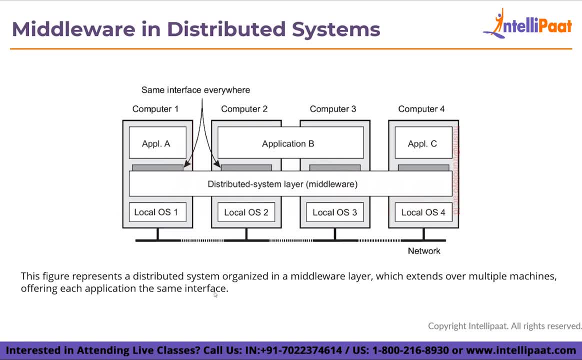 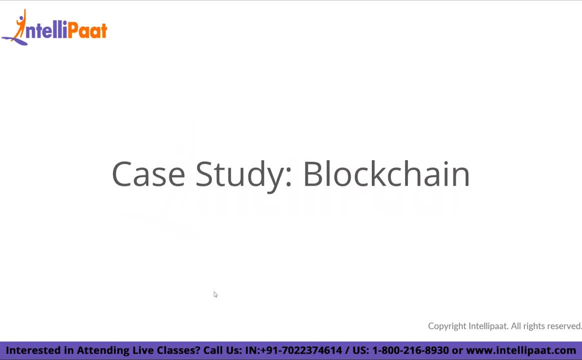 he says that it is the middleware, can be considered as the operating system of a single node. now let us move on to the next topic, which is blockchain. all right guys. now let us take a look at a case study which uses distributed systems, which is blockchain. so blockchain technology. as you might have heard in the news, 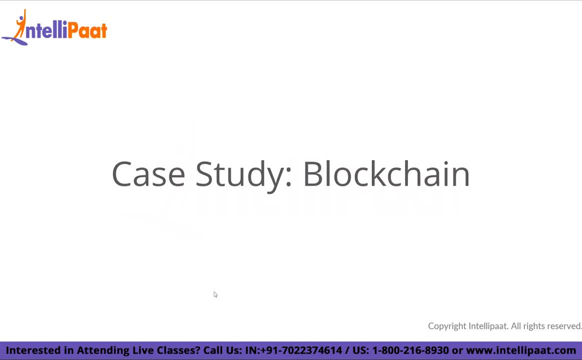 or an some tech forums. everybody are talking about blockchain right now, and it has become famous due to something called as cryptocurrencies. you might have heard about bitcoin, ethereum, etc. so all these cryptocurrencies use blockchain as their underlying architecture. now we will take a look at how blockchain is developed using distributed systems concepts. there are mainly 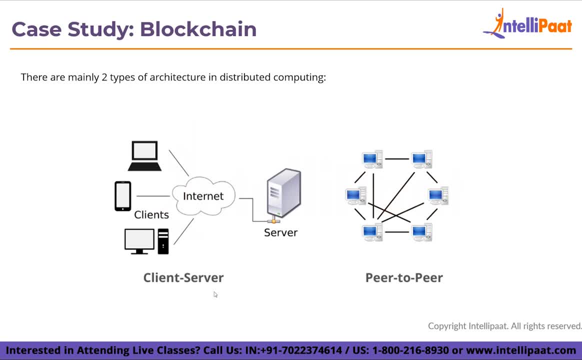 two types of architectures in distributed computing. the first one is the client server architecture. basically, you have one server serving all the clients through the internet, which is called as client server architecture. and then you have peer-to-peer, which also uses internet, but it uses the peer-to-peer network as an overlay network over on top of the internet. 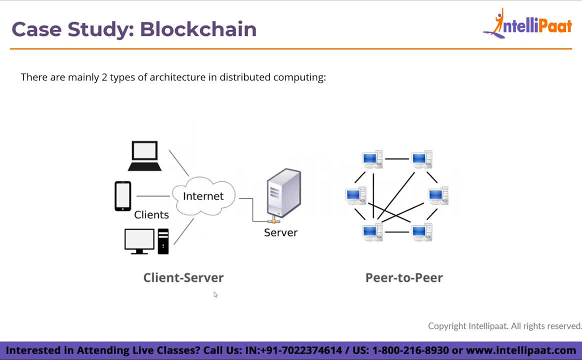 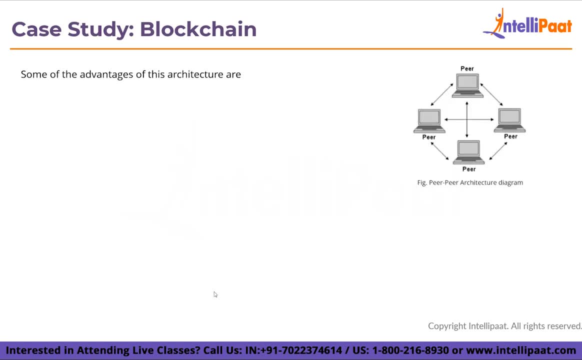 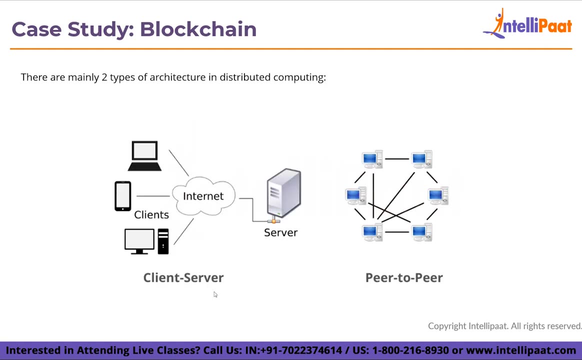 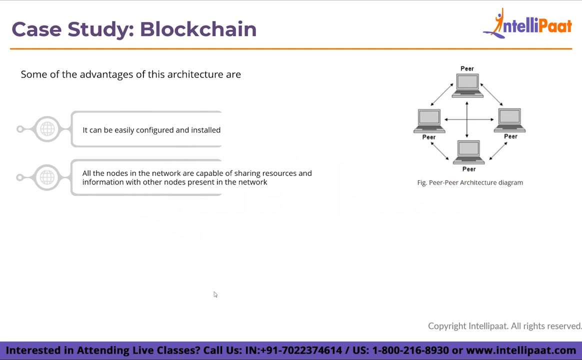 so the second one is that all the nodes in the network are capable of sharing the resources and information with other nodes present in the network. that is, every node is treated as the same and you can communicate with each and every node in the distributed network, even if any node goes. 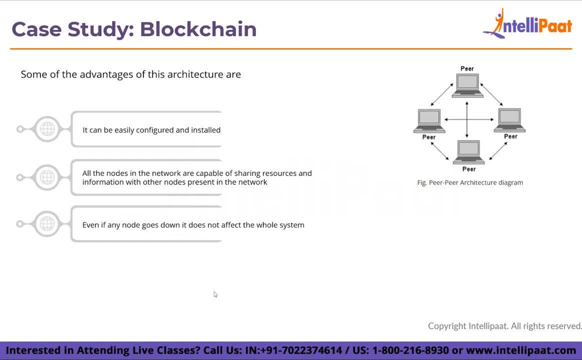 down. it does not affect the whole system. so even if your data is in one node, it will be shared among other nodes, the data will be split up and all the parts of the data will be stored in some of the some or the other node and you can collect that particular. 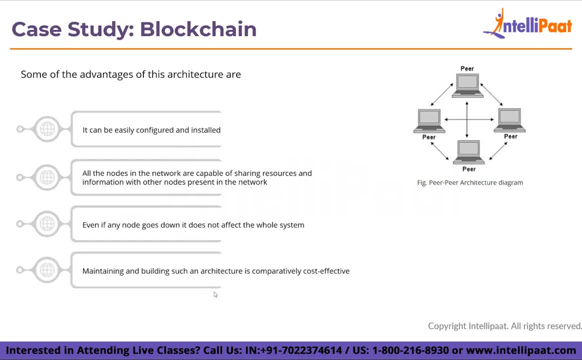 data from all of the nodes in the network. so the fourth advantage is maintaining and building such an architecture is comparatively cost effective. blockchain technology works on the principle of p2p architecture, that is, peer-to-peer architecture, which helps the technology to be more secure and efficient. blockchain technology can be used in many 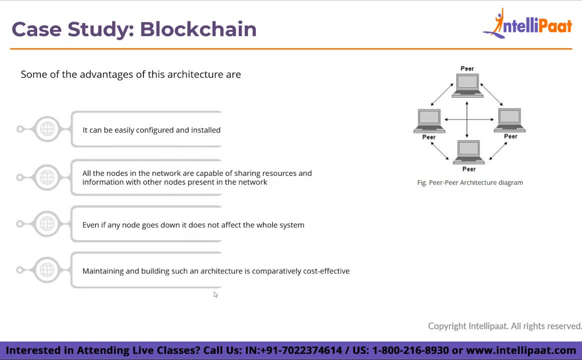 industries, but the main highlight, where it is mostly used, are cryptocurrencies. as I've talked before, a p2p network is central when it comes to doing a transaction within a blockchain. all the nodes can transact with each other in the blockchain. now all the p2p networks are decentralized and that is why blockchain 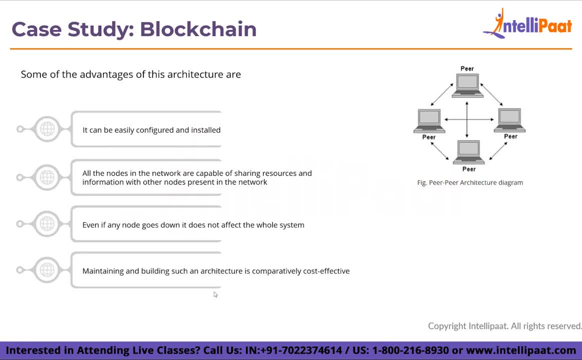 is also known as decentralized applications. this characteristic makes blockchain more secure and hard to hack or break into. in p2p networks, limitations come into the picture when the size of network grows, which results in performance, security and accessibility within the network. Now let us take a look at some of the disadvantages of this architecture. first one is that it 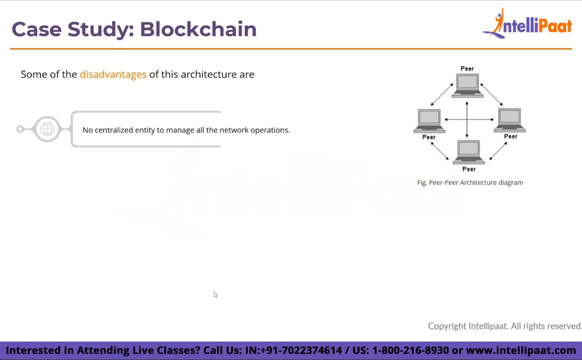 has no centralized entity to manage all the network operations. and the second one is that backup should be done on each computer network. Moving on to the third disadvantage, as any node can be accessed anytime, in order for that network security is applied to each node individually. 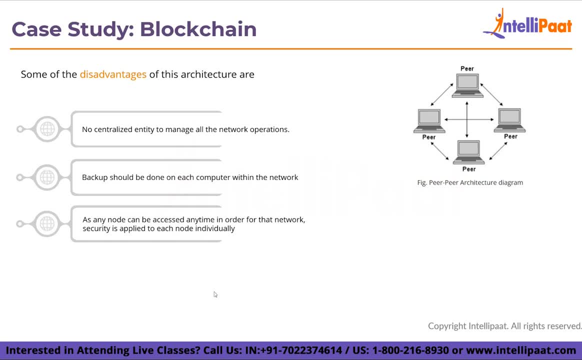 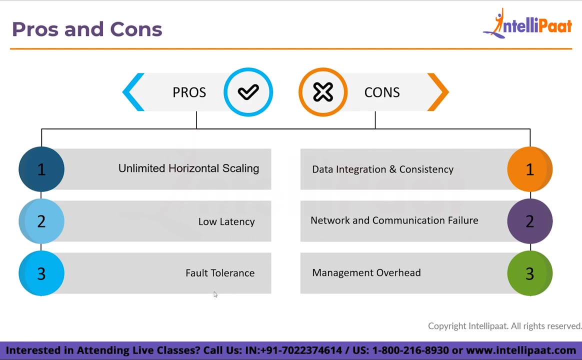 So there is a bit of security concern here, meaning that security should be applied to each of the node individually, but we have workarounds around this disadvantage. Now let us move on to the pros and cons of distributed systems. So, coming to the pros of distributed systems, the ultimate goal of a distributed system. 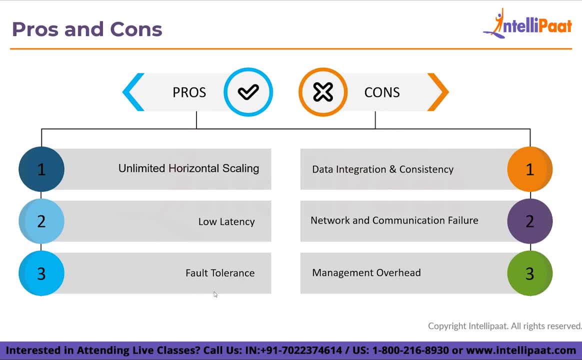 is to enable the scalability, Performance and high availability of applications. So very first pro is unlimited horizontal scaling, which means that machines or nodes can be added wherever required. The second pro is that it provides low latency having machines that are geographically located. 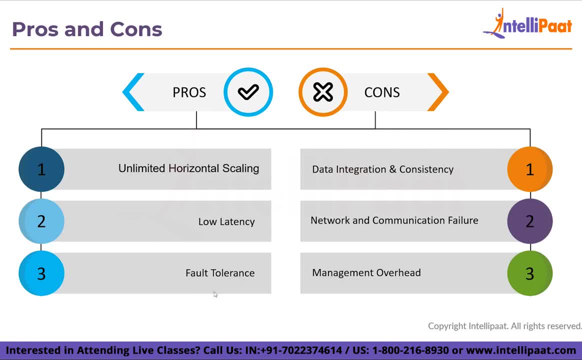 closer to the users. it will reduce the time it takes for the users to be served. The final pro is that it is fault tolerance. If one server or data center goes down, others could still serve the users of that service. Coming to the cons of distributed systems, every engineering decision has trade-offs. 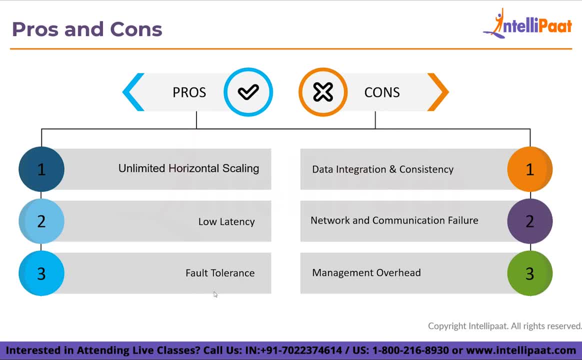 Complexity is the biggest disadvantage of distributed systems. There are more machines, more messages, more data being passed between more parties, which leads to issues with these three things, which are data, integration and consistency. It basically is a very complex system. It basically means that being able to synchronize the order of changes to data and states of 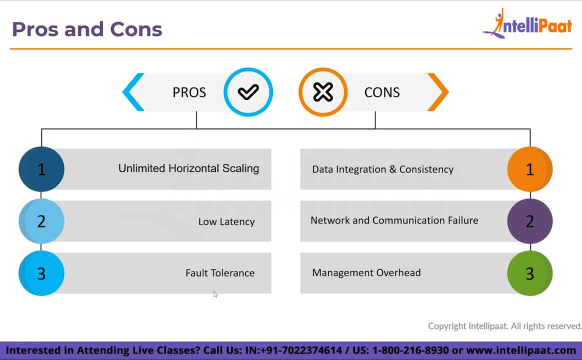 the application And next we have network and communication failure. So messages may not be delivered to the right nodes or in the incorrect order, which may lead to a breakdown in communication and functionality. So maintaining network and communications in a distributed system is very complex. 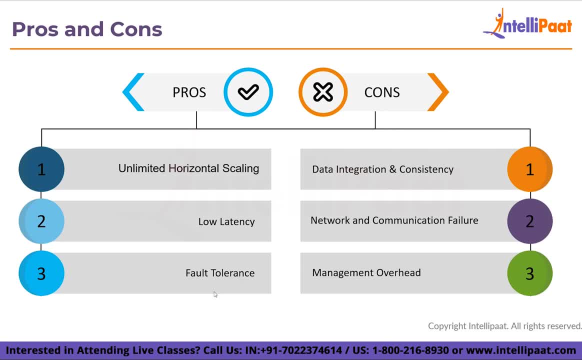 Finally, we have management overhead. So with this con, you have more intelligence, monitoring, logging and load balancing functions needed to be added for visibility into the operation and failures of the distributed systems. So now that the pros and cons are clear, let us move on to the last topic of this video.